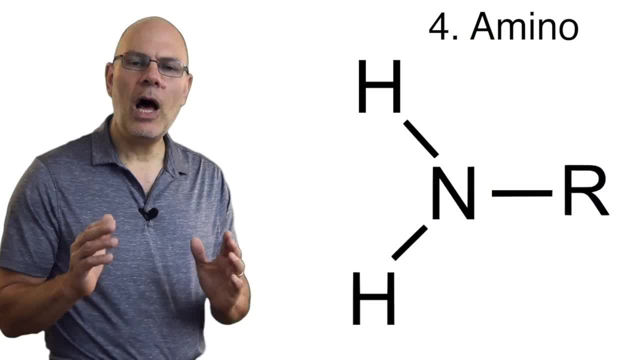 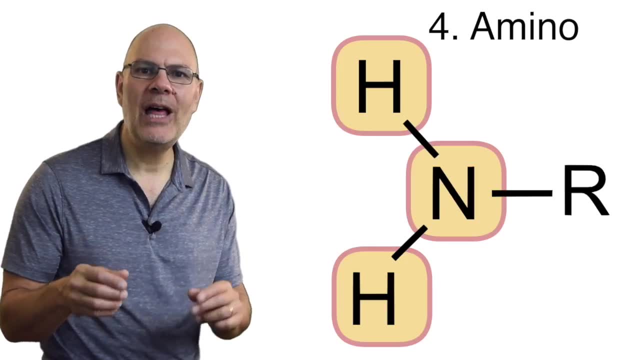 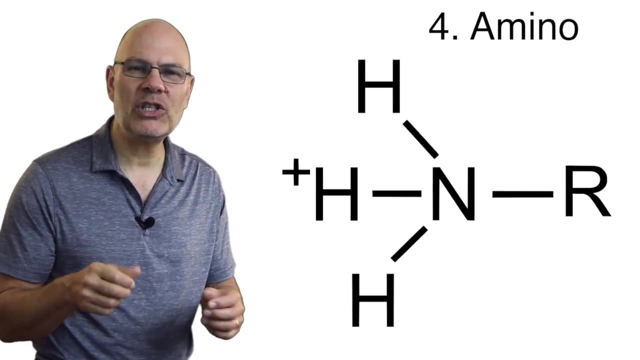 both the non-ionized and the ionized forms. Amino groups consist of a nitrogen attached to two hydrogens. When you connect an amino group to a molecule, that makes it a base, because the amino group in water will pick up a proton from the solution, increasing the pH. That makes the amino group look like. 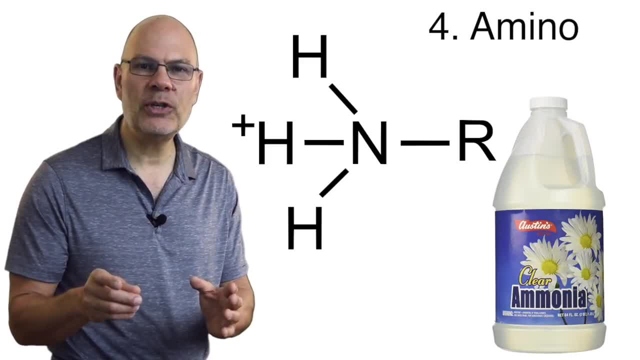 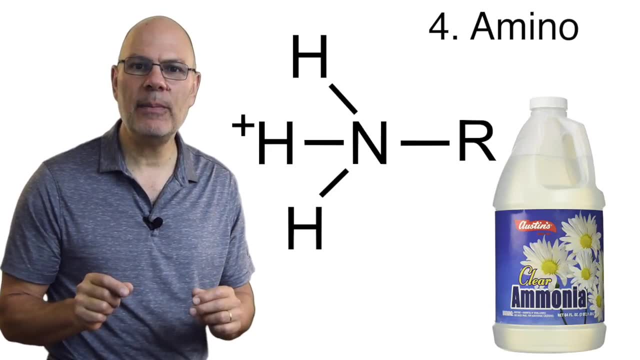 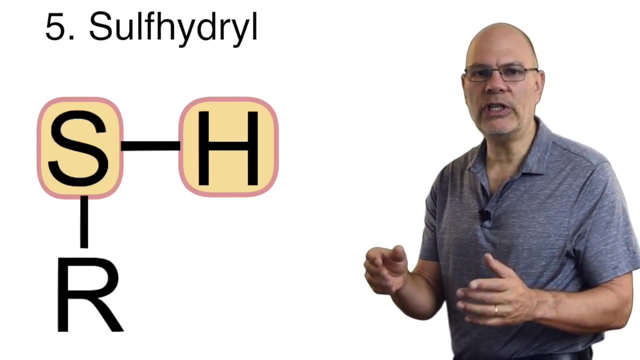 this. It'll have three hydrogens and a positive charge. Just remember that amino sounds like ammonia. Ammonia's formula is NH3, and it's a base, just like a hydrogen. Sulfhydryl groups consist of a sulfur bonded to a hydrogen. Sulfhydryl groups are important. 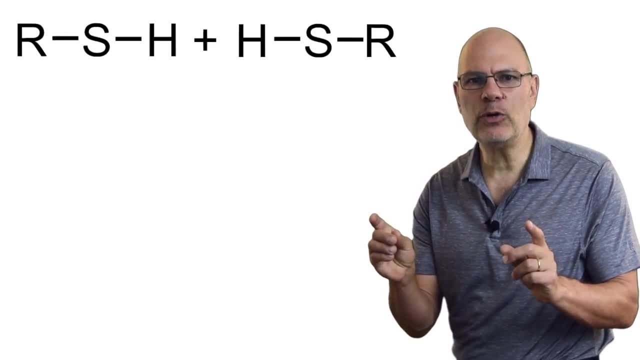 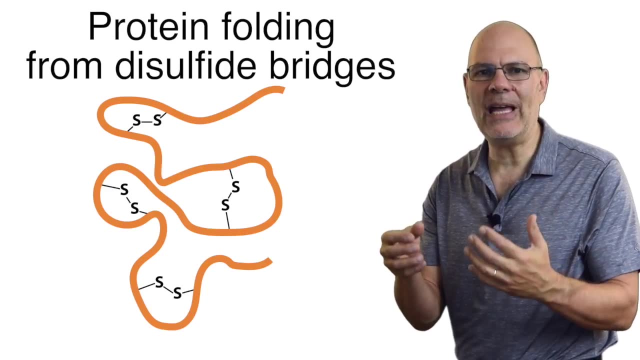 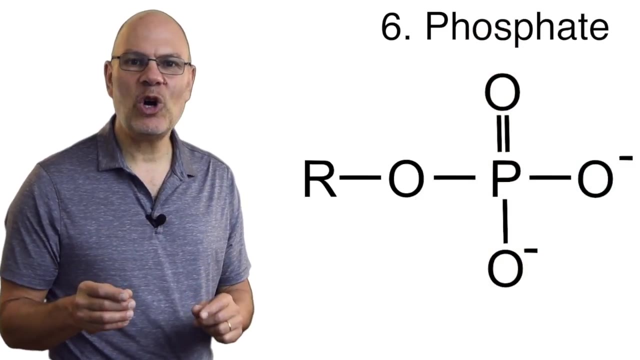 in determining the shape of proteins, because when two sulfhydryl groups become close to one another, they can form a disulfide bridge That creates turns and bends in a protein chain and that determines the protein's overall shape. A phosphate group is a negatively charged ion that consists of one phosphorus atom surrounded. 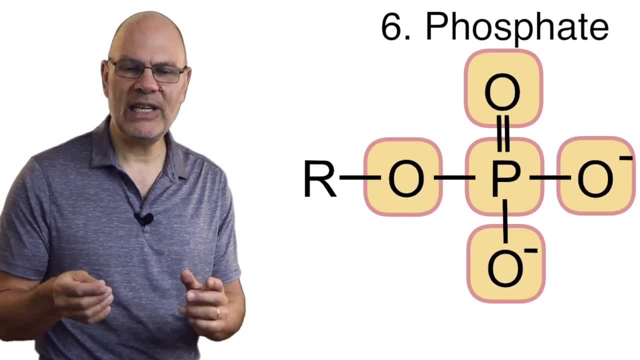 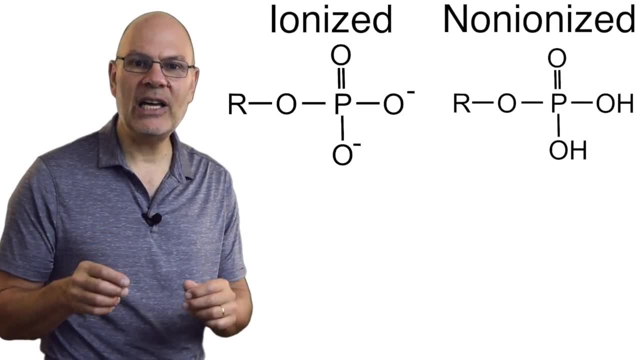 by two oxygen atoms. Phosphate groups make molecules acidic. You should be able to identify this ionized form of a phosphate group, which is what's found in cells, this non-ionized form which you might find in a textbook or on a test. 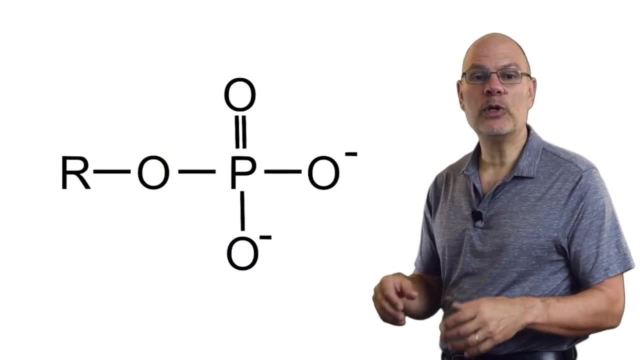 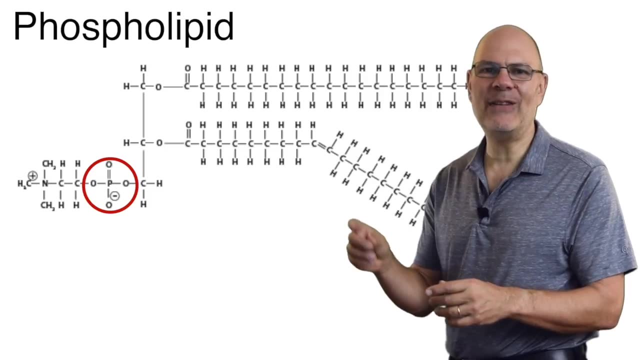 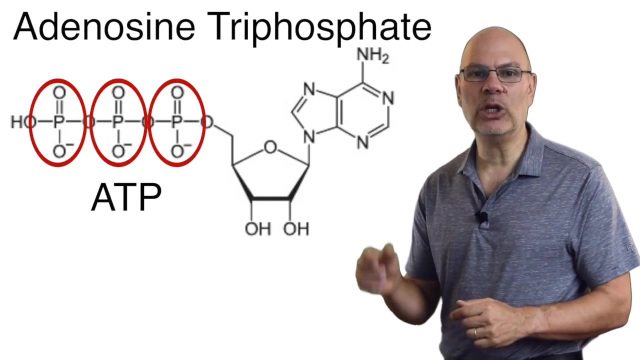 and phosphate's chemical formula, PO4.. Phosphate groups are incredibly important. Here are phosphate groups making up the backbone of DNA. Here are phosphate groups in the head of a phospholipid, the key molecule in cell membranes. Phosphate groups in life's key energy molecule, ATP. 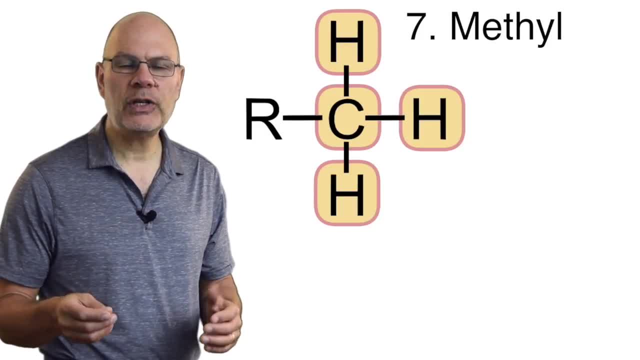 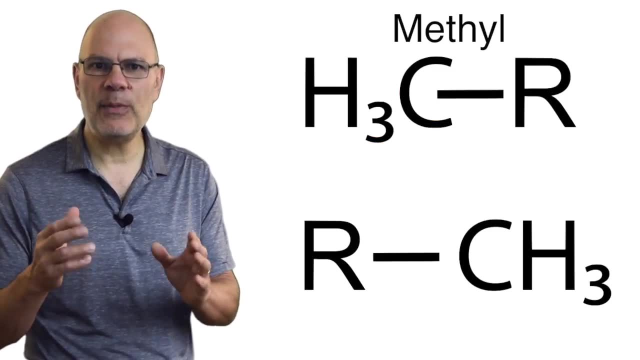 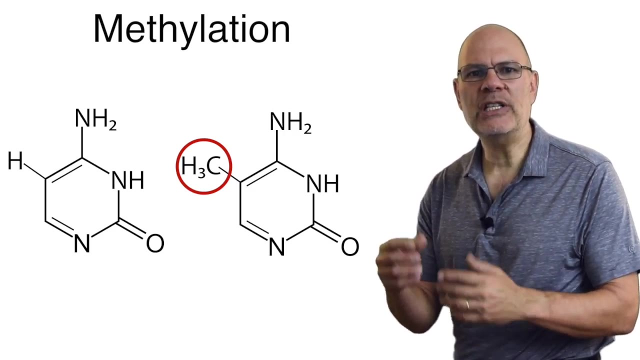 A methyl group is a carbon connected to three hydrogens. If you know the natural gas, methane, then a methyl group is very easy to identify. You'll also see methyl represented by its empirical formula in one of these two forms. Adding methyl groups to a molecule is called methylation and it creates a non-polar region. 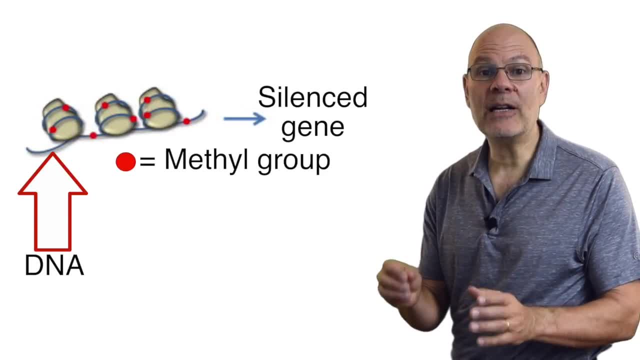 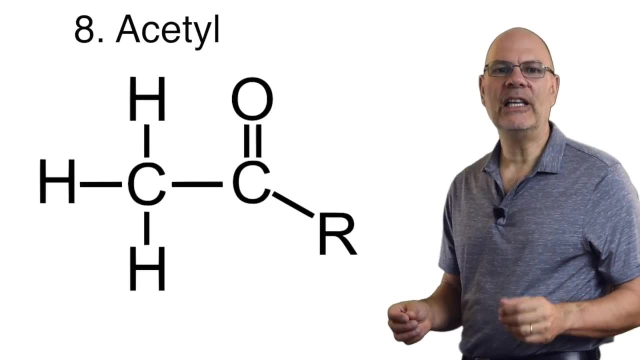 where the methyl was added. Cells use methylation to modify DNA. Methylated DNA won't be transcribed in the cell. This is essentially turning the DNA off. Finally, here's an acetyl group. It consists of a methyl group bonded to a carbonyl. 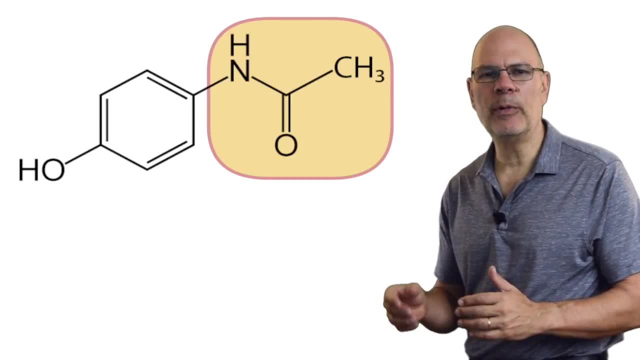 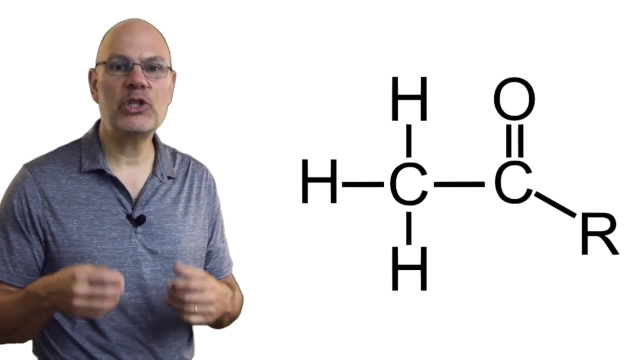 Take a look at this molecule. This piece over here is the acetyl group. This molecule is known as acetaminophen, better known as Tylenol. Adding an acetyl group to a molecule is called acetylation. Later in the course, when we